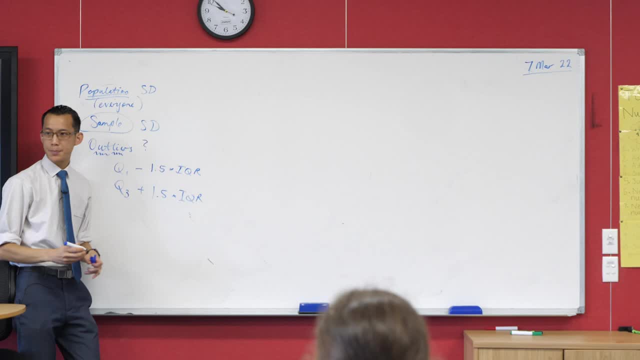 one and a half times the interquartile Range. Okay, Now I'm coming back to Sebastian's question. He said: what even is standard deviation? Okay, it's a way actually to understand how spread out the data is, and it helps us. 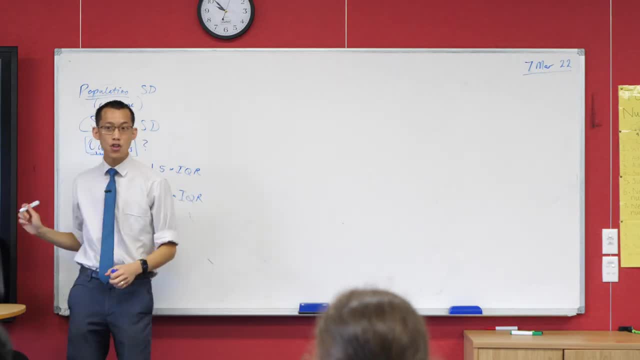 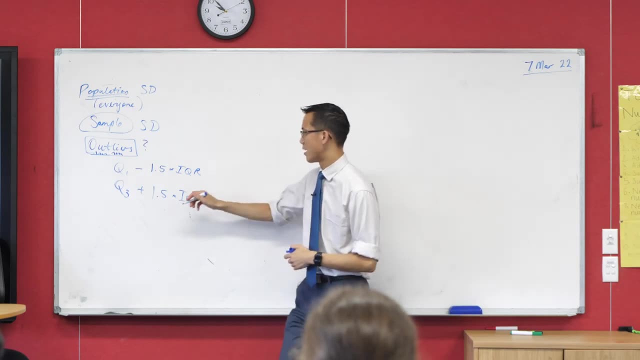 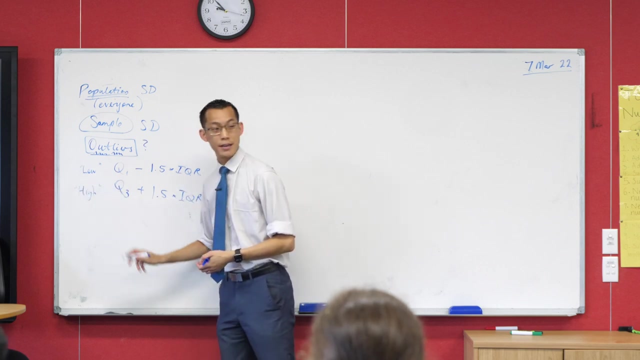 actually unpack this a little better, because this is not the only definition or not the only way to calculate an outlier. You can say: these are the, you could call these the low outliers and you can call these ones the high outliers, If you like. anyone who's. 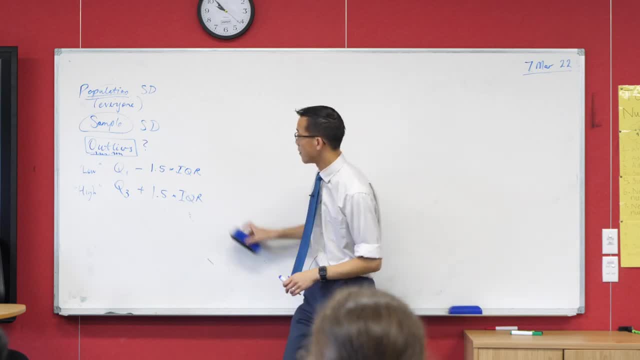 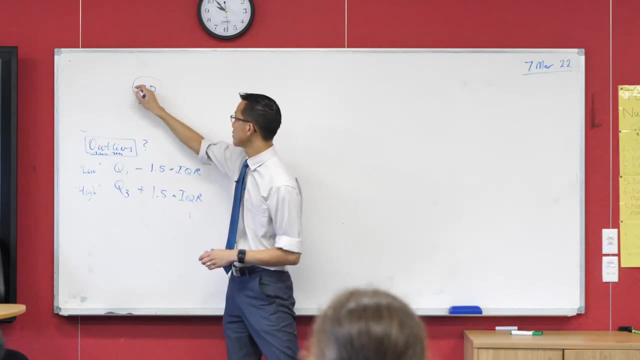 outside of this. okay, But we can actually use- let's not worry about this for now. We can actually just talk about this as one big concept. We can actually use the standard deviation to help us define what an outlier is, but it works in much the same way as going low and going high. So 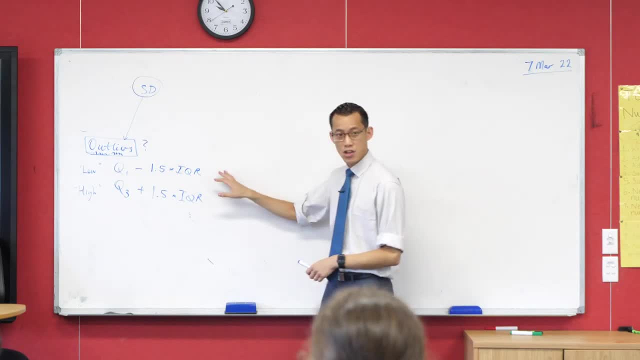 you've probably got this written, like in last week's work, but can you write it for me again, because I want to define it in a different way in terms of the standard deviation, and we'll use this set of data to help us, okay. 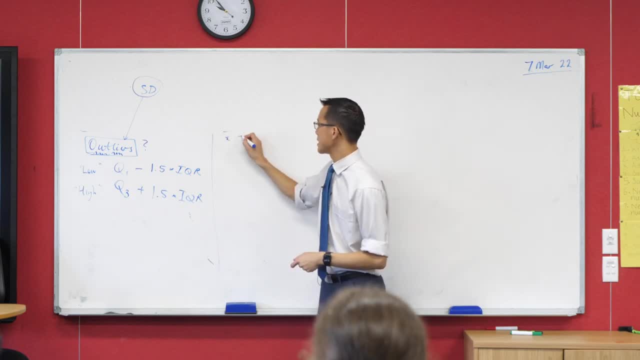 Can you remind me again, For this set of heights, we've got a mean, an x-bar of what was it? 170, 170? what 0.6?? And then we've got a standard deviation, or you can actually use a sigma. 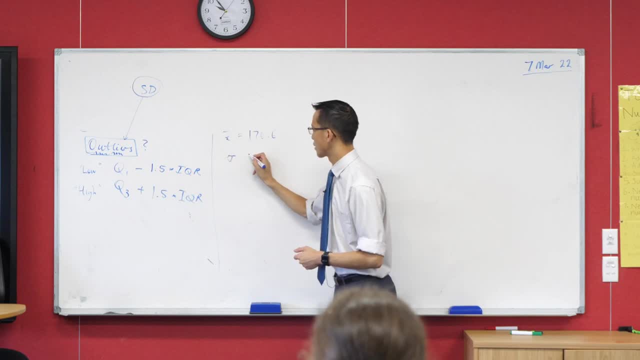 that's a Greek letter like so, except my whiteboard marker's not doing great, And I think from memory you said it was 10 point something, right, 10.2?. Thank you very much. Okay, now what we can do is use this same idea here and say: well, let's just go like. 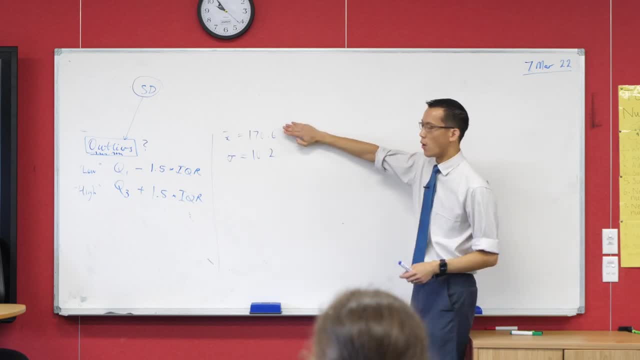 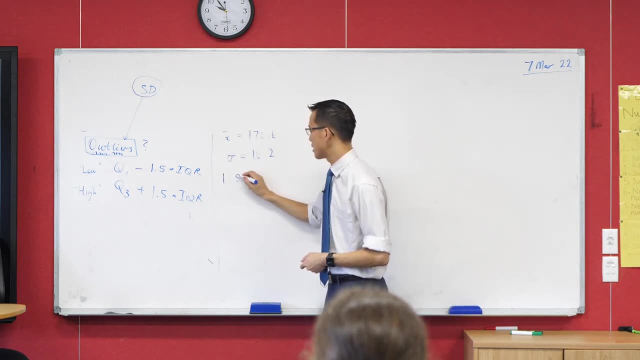 up and down. okay, We would say, if you are one standard deviation away from the mean, so this is a range right. So we would say let's call this one standard deviation within the mean. So what I'm doing is I'm using that x-bar and I'm saying: let's go down and let's go up and see. 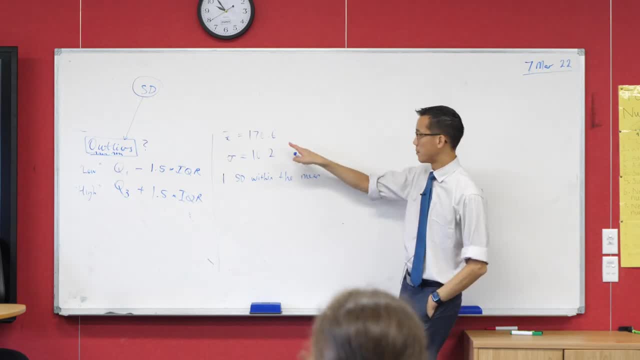 what range we get. okay, You're going to need your calculator for this one. If I go down one standard deviation, so 170.6,. take away this. it's easy numbers for now. In this case it would be 180.4, right? I didn't calculate these beforehand, I'm just hoping that I'm doing this right on the. 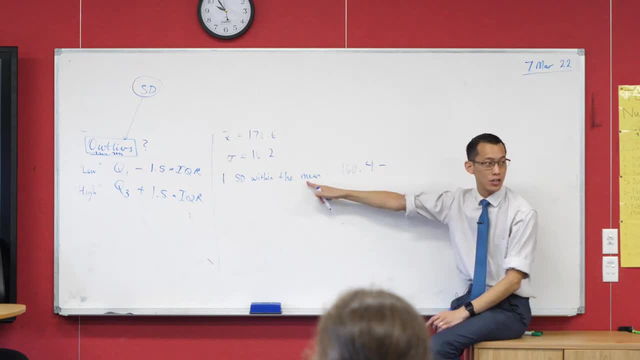 easy numbers. There's my lower boundary for one standard deviation away. How high do I go? If I add a standard deviation, how far will I get 180.8.. Thank you, whoever designed this question, for giving us easy answers. Okay now, this is within one standard deviation of the mean. 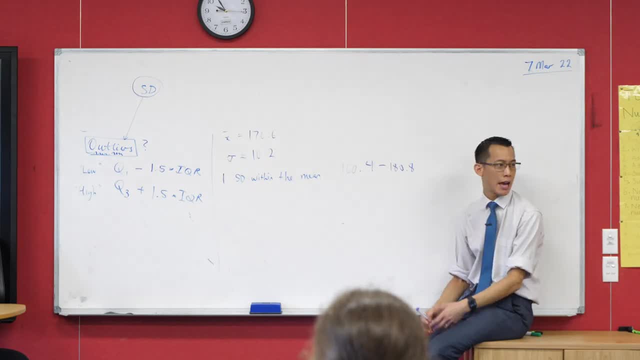 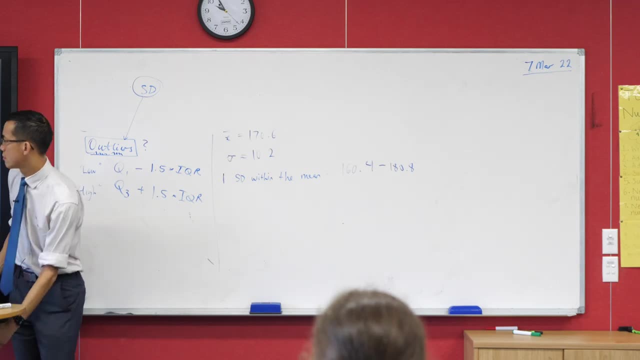 Have a look over again at the data. How many people, or how many U12 students, are within this range? Have a look. We've only got the classes, I know, but check it out Like let's just treat that as. 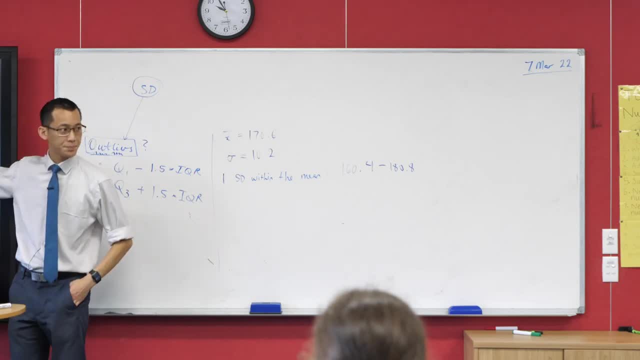 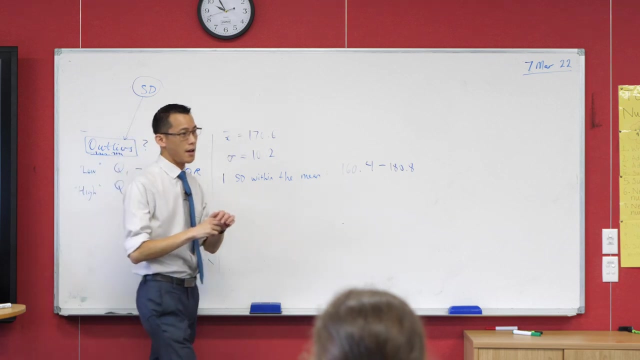 160 to 180.. How much of the data have we captured? A lot, right, If we call this 160, right down to 180, it's here. yeah, Can you go ahead and do a quick calculation for me: 27,, 31,, 12,, 15.. I don't. 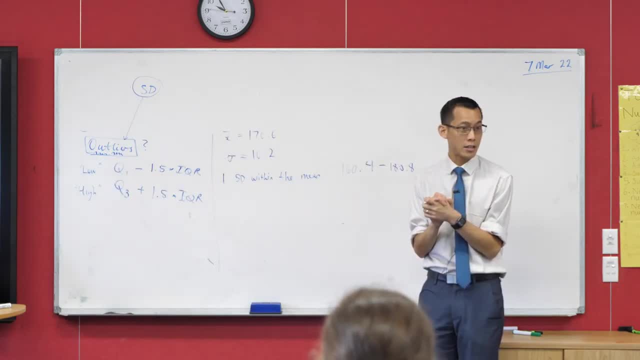 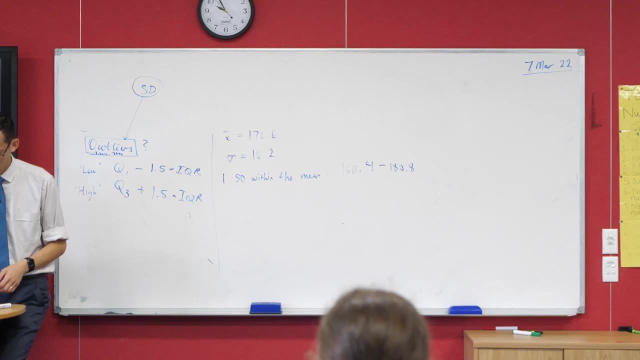 even know what the total number of students is. but you can help me work that out as well using this. You can't quite recall. You should be able to go to shift 1, back to variable, and then I think n will tell you the total number. How many people have you got in there? How many again? 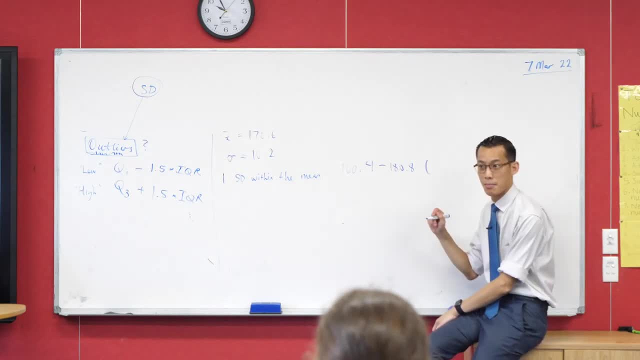 Like, actually tell me how many people we have in here. 85,, just in this range, okay, 85, and what's the total number of people, What's our population for this? This is 85 out of how many Someone? 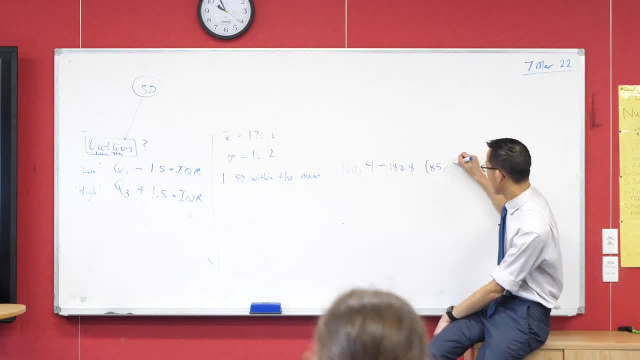 gone. Don't add it up. Your calculator's already done it right: 145,. thank you very much. Okay, so this is more than half of the people. More than half of the people are within one standard deviation. okay, Let's go. 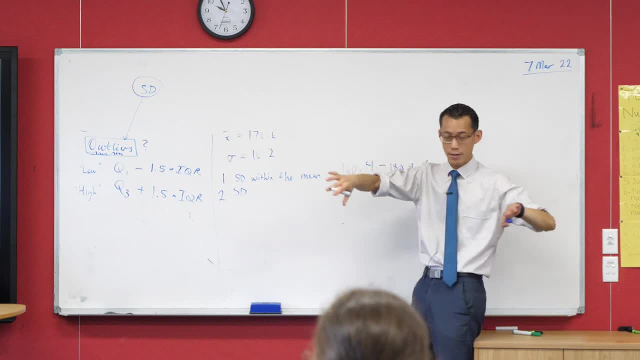 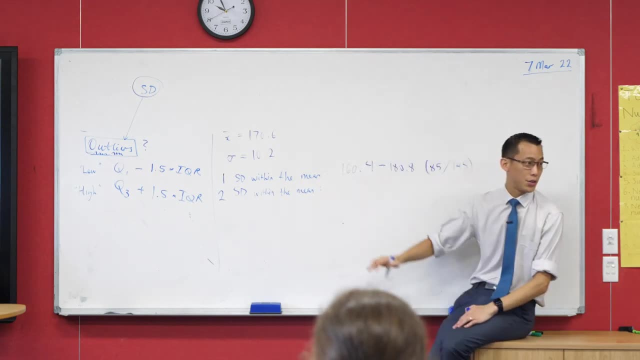 further If we go two standard deviations away, two standard deviations within mean. So now I'm going to start from x bar again, but this time I'm going to subtract 20.4, and then I'm also going to add 20.4,, right? So this new range will be: 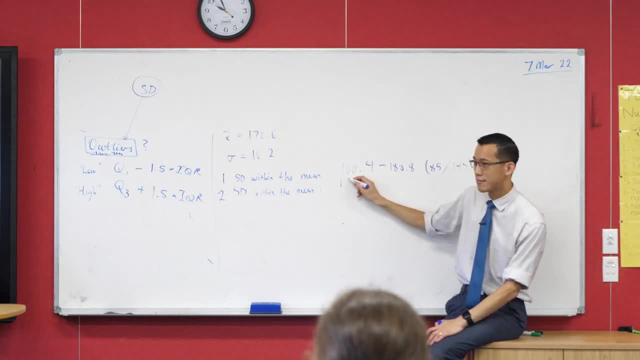 I know it's Monday morning. you guys can do it right: 150.2,, 150.2, all the way up to it's this plus 10.2, isn't it? That's an easy way of doing it, So that'll be 191.0,. okay, Now I'm going to. 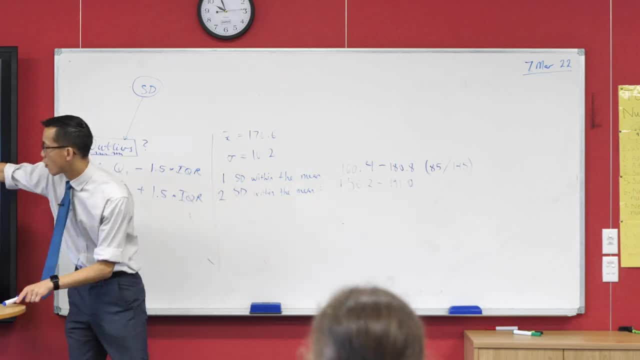 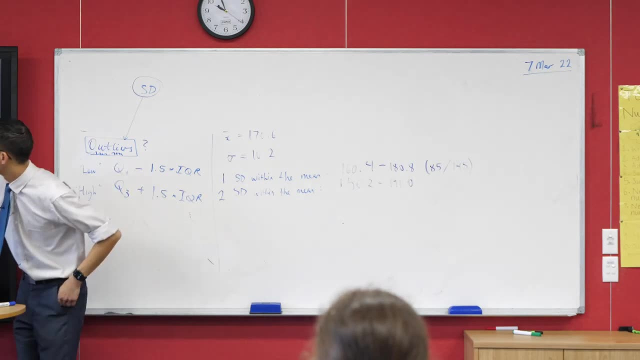 ask this question again. We're going further out, We're starting again from the middle. it's around here and we're expanding right. So this is going to be well, let's see 150, so in fact that goes all the way down to all of these people, and then we 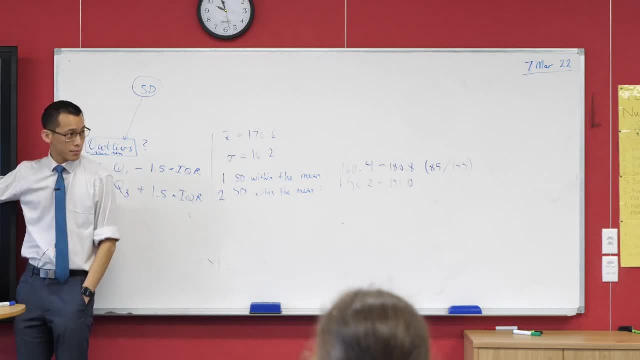 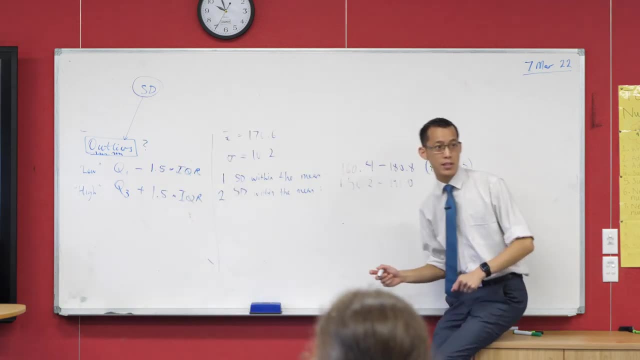 go up to 191. So actually I guess we'd call there How many people is that? It's everyone except for three. yeah, So what did you tell me? the total was 145? So what's this now How many? 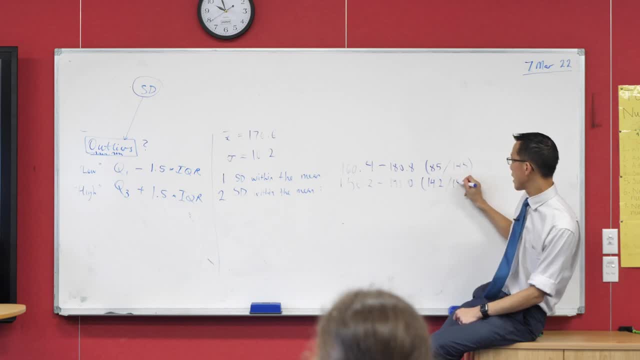 people, 142 out of 145,. okay, Now I don't need to go a third standard deviation, because I would capture everyone. yeah, But this is well actually you can go around and see if there's ahead and put that in your calculator. what percentage is that? 98 percent, 97.5. what do you got? 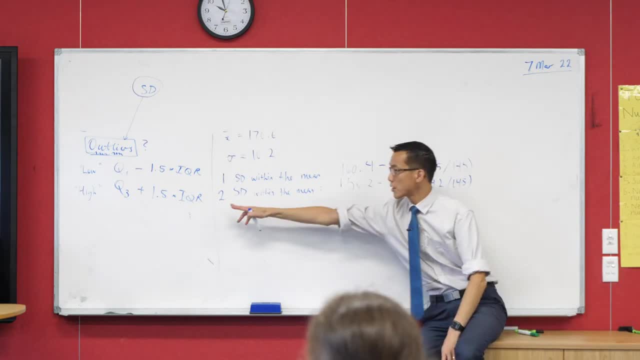 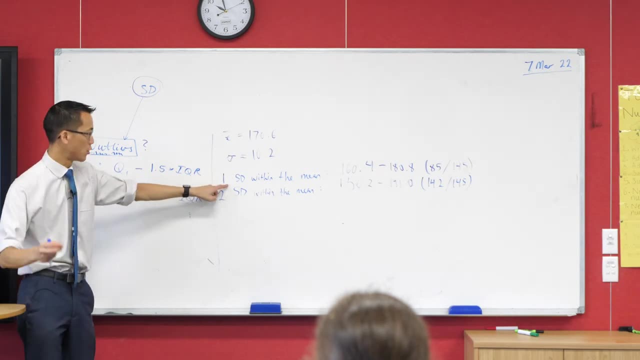 oh the wait, these numbers here, yeah, so okay, great question. in much the same way that we used interquartile range as a measure of spread right, standard deviation is just like a better measure of more accurate one. so in much the same way here. i went from a number and then i added the. 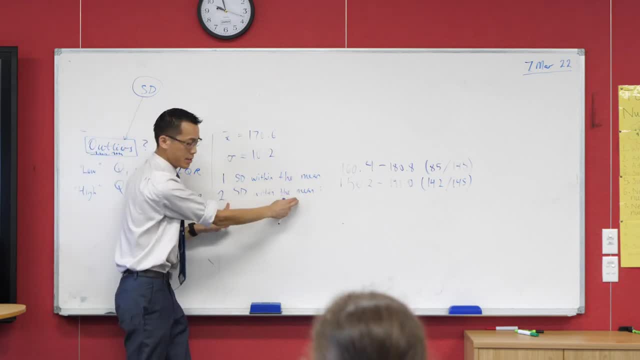 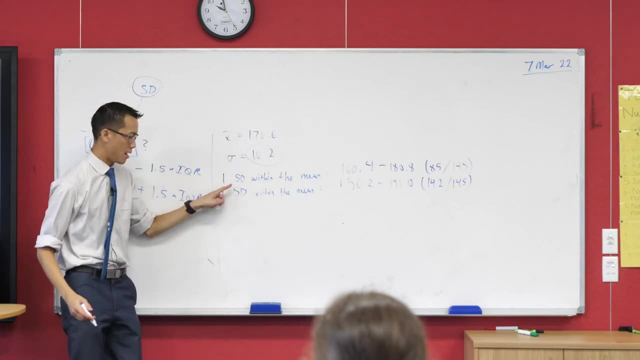 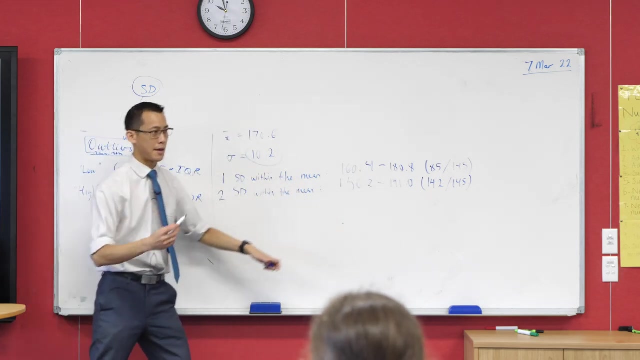 interquartile range. here i'm going from the mean in both cases and i'm adding some number of standard deviations. in this case i added one of them which took me up to 180.8 from here. in this case, i added two of them which took me higher. sorry for the bad marker. okay, now i'm going to 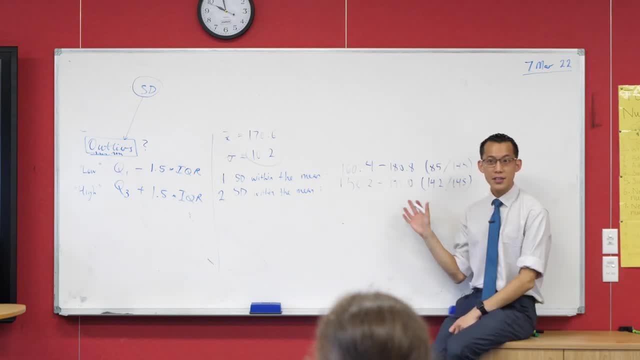 close this off and then we're going to have a look at some different data. this idea of using the standard deviations to work out outliers we can see within two standard deviations we pretty much we almost can't capture everyone. okay, the technical definition for low or high outliers using the standard. 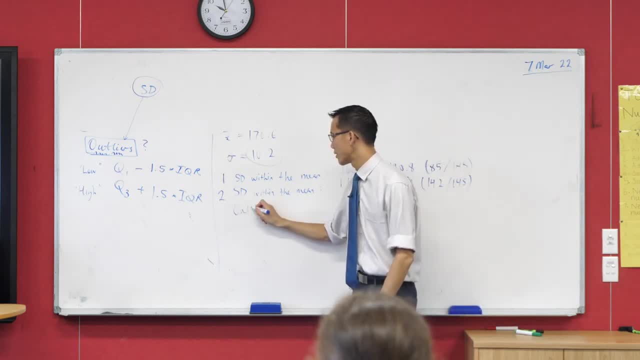 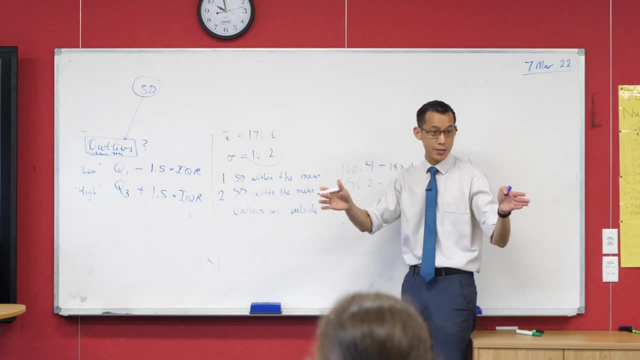 deviation is outside or outliers are outside, again because we said they lie outside two and a half standard deviations: 2.5. this thing is going to drive me crazy. maybe i'll just write it. the rest, um on my ipad: outside: 2.5 standard deviations. if you've got someone who's outside. of that, you're going to get 7.5 standards, because then you're going to write all the deviations right over here. lol, every time i get 6 i write less than instead of 7, so that means you constantly lengthy myinishet. here is the smallest only code you can write to everybody, except you're bringing.